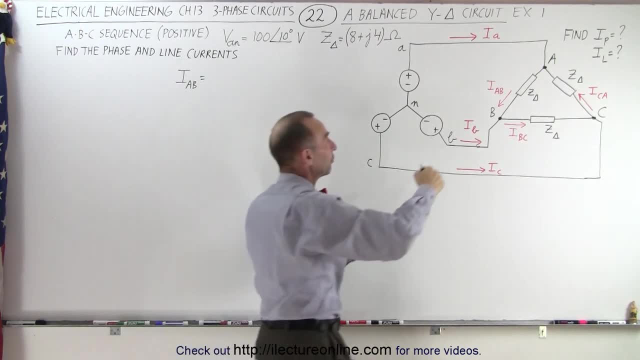 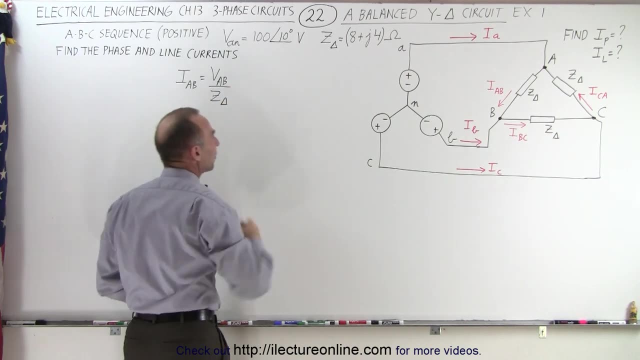 the current must equal the voltage divided by the impedance, and it will be the voltage from A to B divided by the impedance. And the voltage from A to B is the same as the voltage of A to B here in the source. So we can. 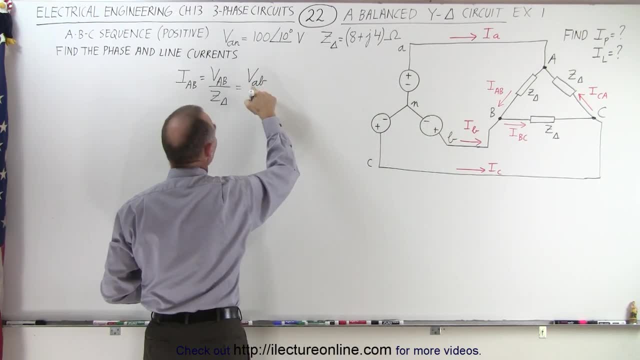 write this as Vab, which means the line voltage divided by the impedance. Now we're not given the line voltage, we're given the phase voltage, and they differ by a magnitude of the square root of three. So in other words, the line voltage equals the square root of three times the phase. 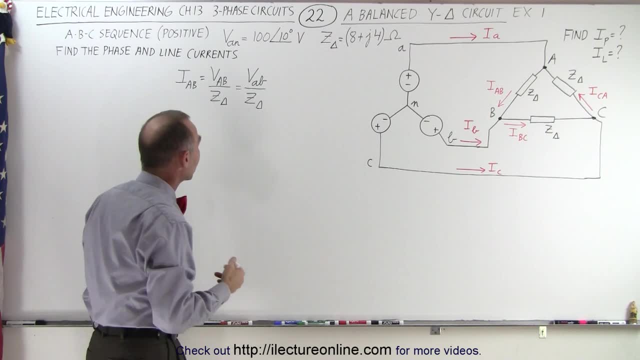 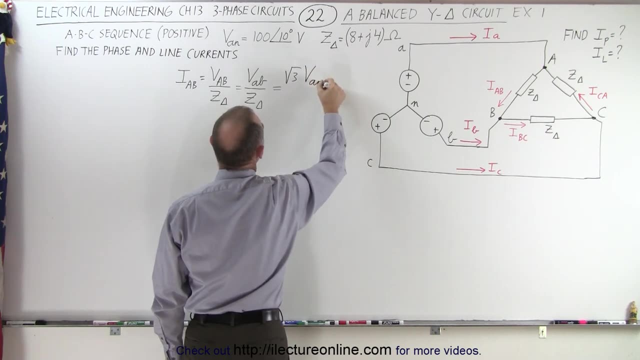 voltage, and it also differs by a phase angle of plus 30 degrees. So that means that this is equal to the square root of three times Van, plus a phase angle of 30 degrees, and we divide that by the impedance. So now we're ready to plug in the numbers. So this is equal to the square root of: 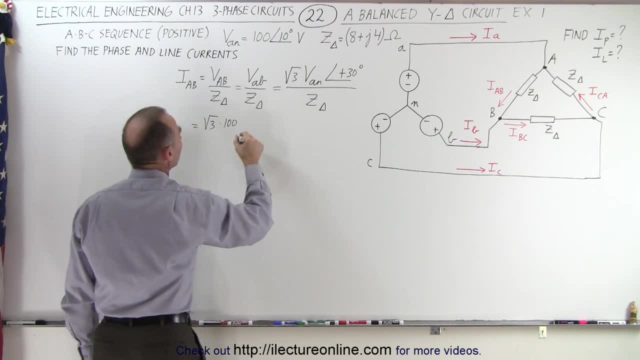 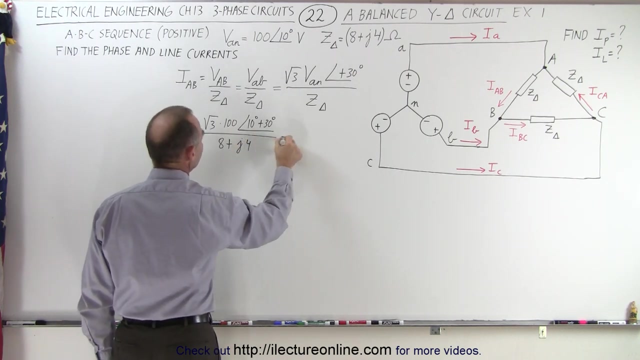 three times 100, with a phase angle of 10 degrees plus the phase angle different between the phase and the line voltage of 30 degrees, and we divide that by the impedance, So this is equal to the voltage divided by eight plus J4.. All right, so let's go ahead and find the values of that. So for 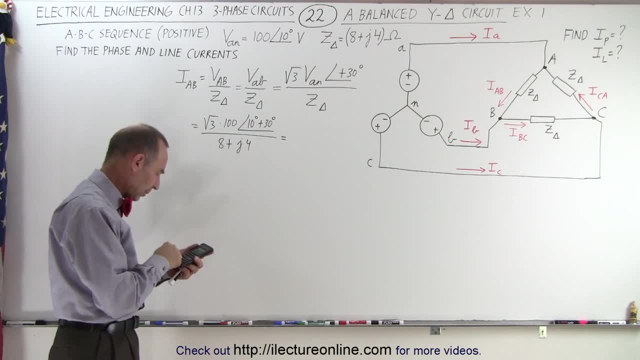 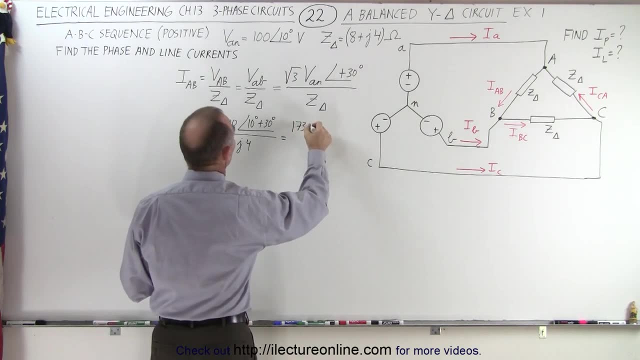 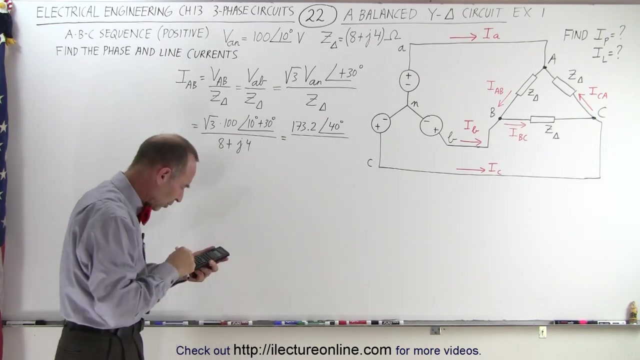 the numerator, we have a magnitude of. take the square root of three times 100, that's 173.2.. We'll do 173.2 volts with a phase angle of 40 degrees and we divide that by a magnitude of. 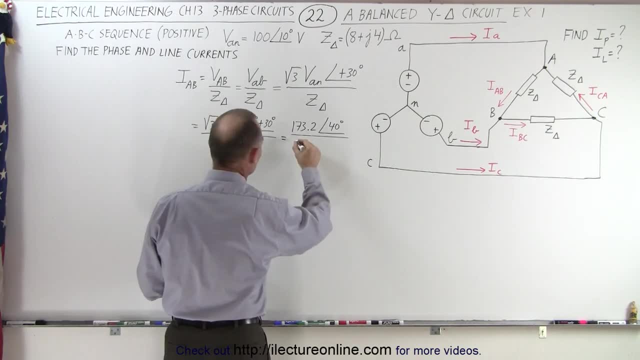 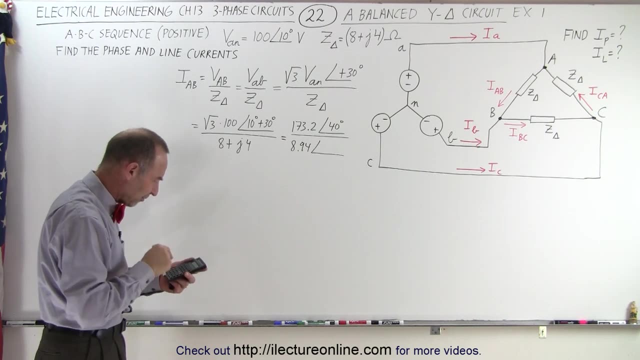 let's see that would be 80,. take the square root, that's 8.9.. 8.94, 8.94 with a phase angle of four divided by eight, that's 0.5.. Take the inverse tangent of. 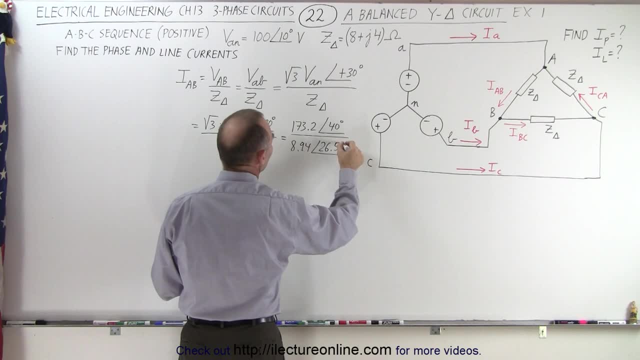 26.565 degrees. 26.565 degrees. There we go. We don't need to write it, Let's just write it as 57 degrees. That's better. There we go, And calculating that, so we have 173.2 divided by. 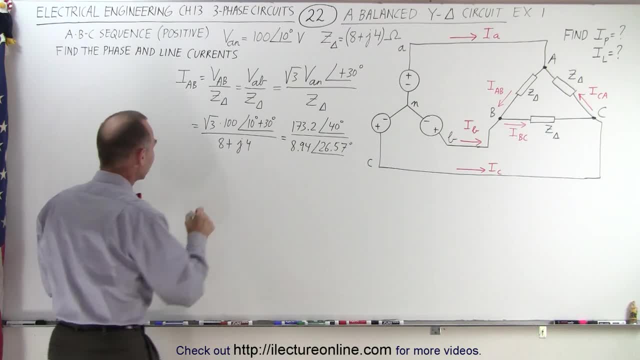 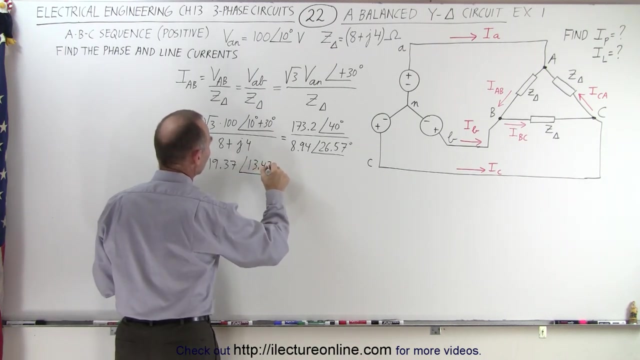 8.94.. It gives us 19.37.. That's equal to 19.37, with a phase angle of 40 minus 26.57.. That's 13.43 degrees And of course that's in terms of amps. That's the first phase, current IAB. All right, so that gives us the 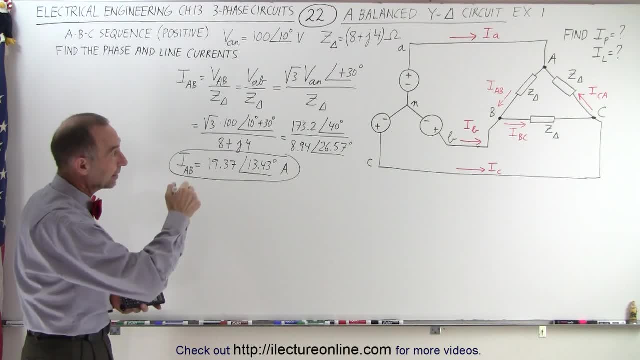 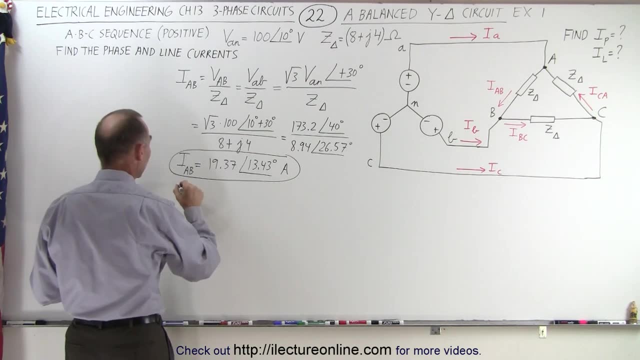 magnitude and the phase angle of that phase current. Now to find the other two phase currents, IBC and ICA, we simply subtract 120 degrees from each of those, So that means that IBC is equal to 19.37, with a phase angle of 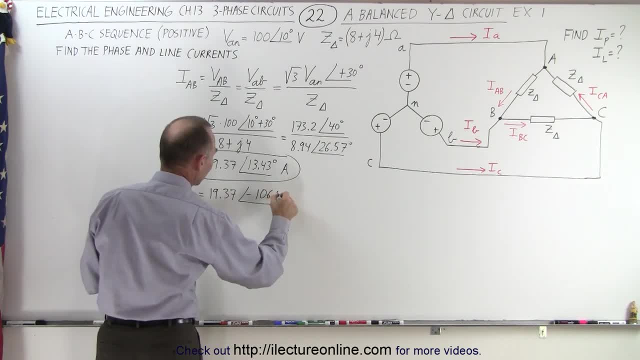 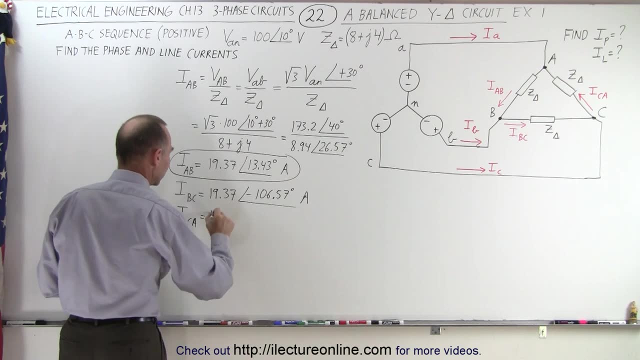 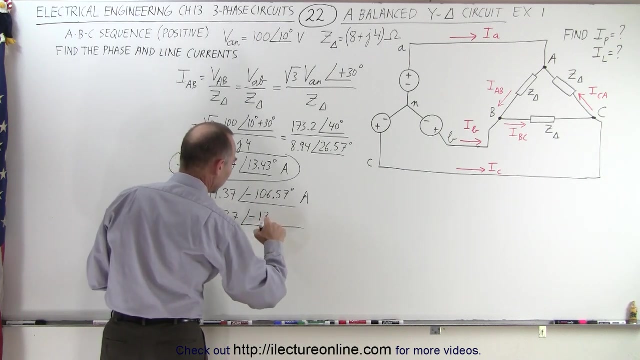 106.. That's minus 106.57 degrees. Of course that's in amps And ICA, the third phase, current 19.37, with a phase angle of minus 100 and oops, not 36.. That would be. 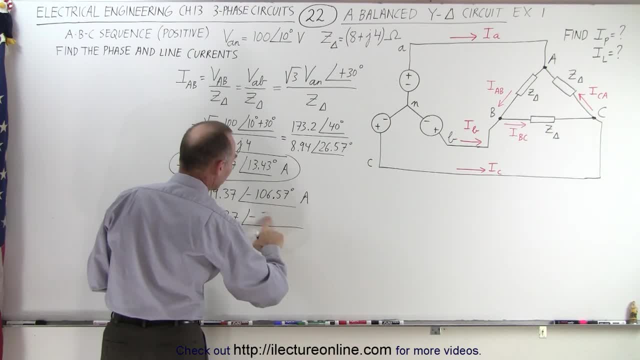 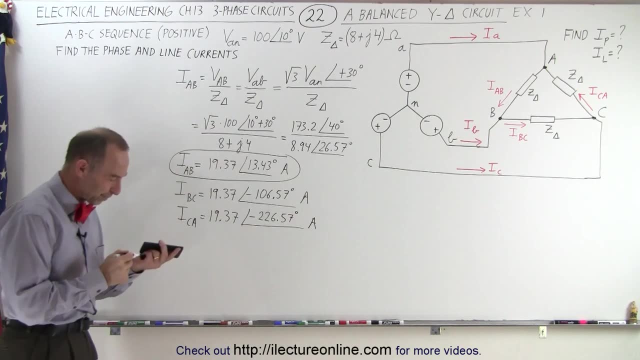 26. Whoa, whoa, whoa, whoa, Minus 120,, minus 226.57 degrees, And also in amps right there. So those are the three phase currents: IAB, IBC and ICA. 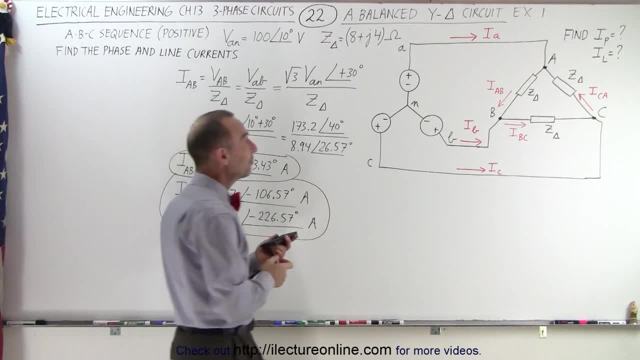 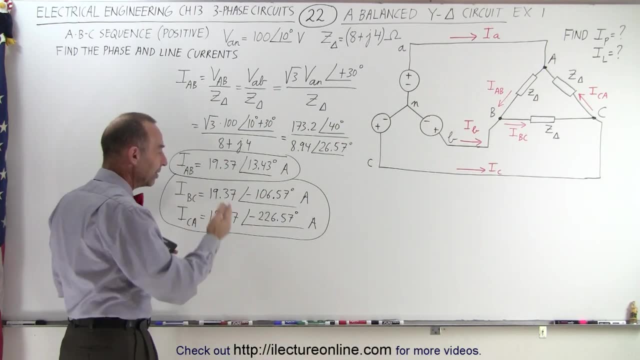 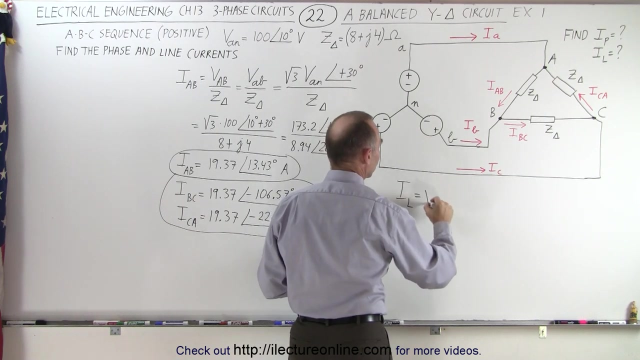 From that we now need to find the line currents, the currents that feed the load: IA, IB and IC. Now, there again, there's a difference between the magnitude and the phase. We know that the line current is equal to the square root of three times the phase current, with a 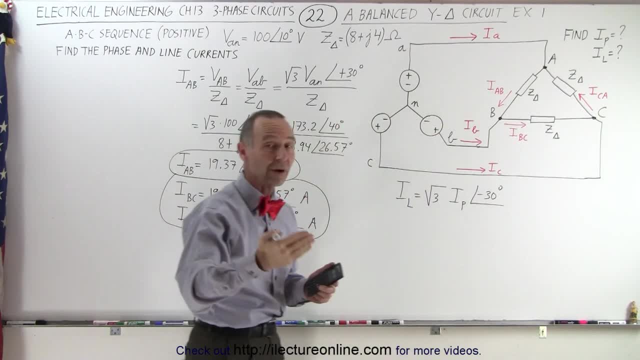 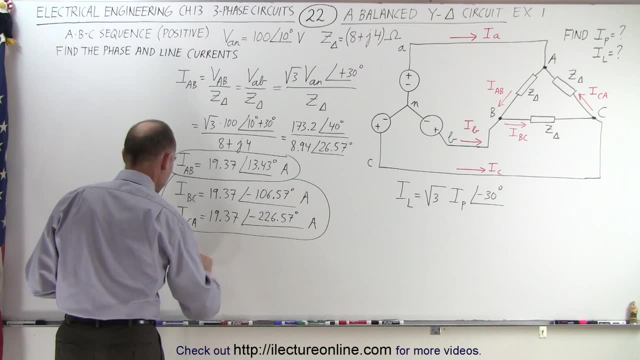 shift in the phase of a minus 30 degrees. that means we subtract 30 degrees on the phase angle and we multiply the magnitude by the square root of three, which means that ia, the line current, is going to be equal to the square root of 3 times i, a, b, but with a shift in the phase of minus 30. 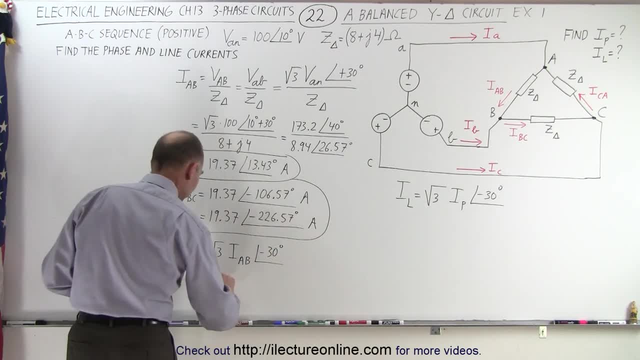 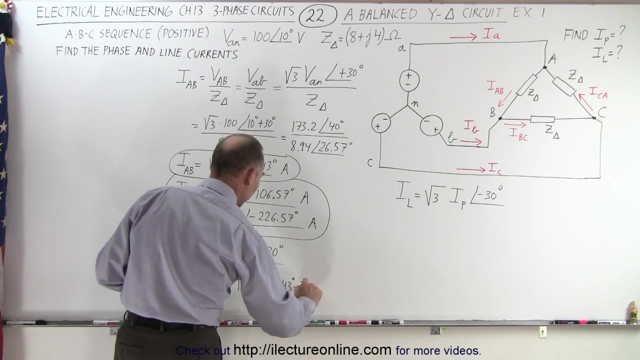 degrees, and so when we plug that in, that's equal to the square root of 3 times i- a- b. let's see here that would be this one: 19.37, with a phase angle of 13.43 degrees minus 30 degrees. okay, what does?